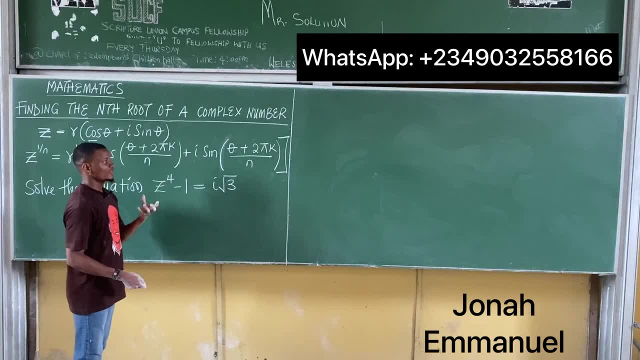 in terms of radians. So if you want to get your value in terms of degrees, simply replace pi by what's there: 180 degrees. Alright, we'll take a sample problem and see how this works. So example number one: it says: solve the equation. 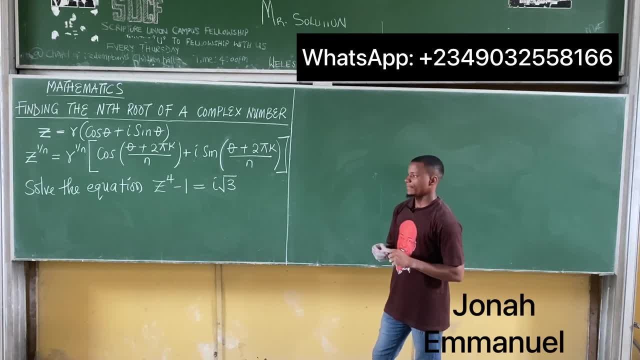 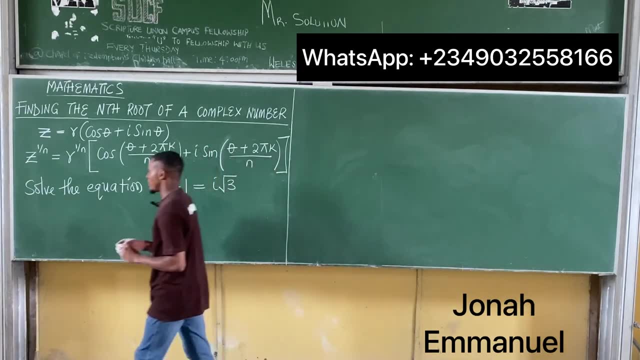 z to the power. 4 minus 1 is equal to i plus root 3.. For this case here, my first task would be to move this one here over here. That means z to the power 4.. So it means that z to the power 4. 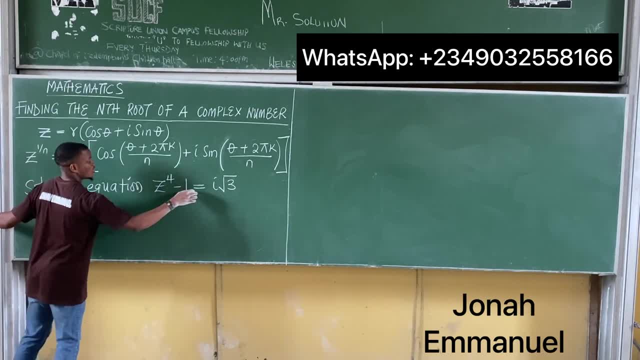 here is equal to minus. 1 comes over here becomes plus 1.. That becomes plus 1.. That's i root 3 plus 1.. Rearranging this: we know we should have the root part before the imaginary. So that would be equal to the real part first, 1 plus the imaginary part. i root 3.. So it means that 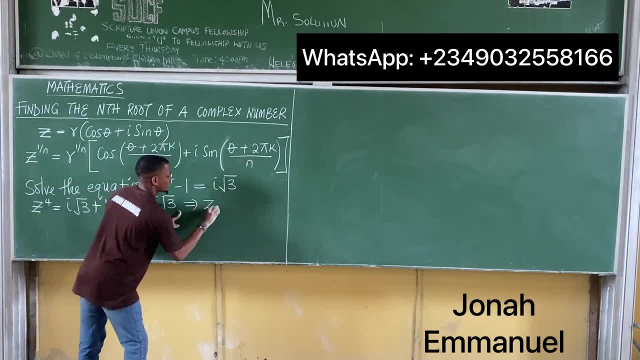 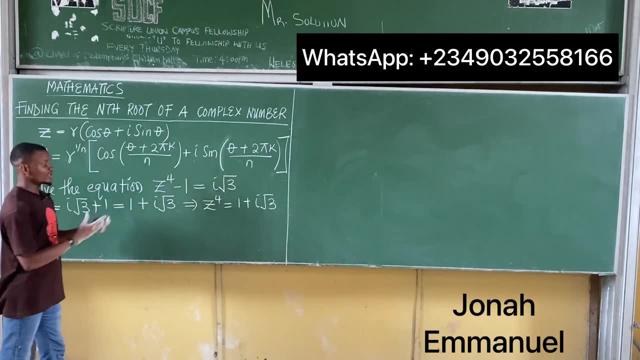 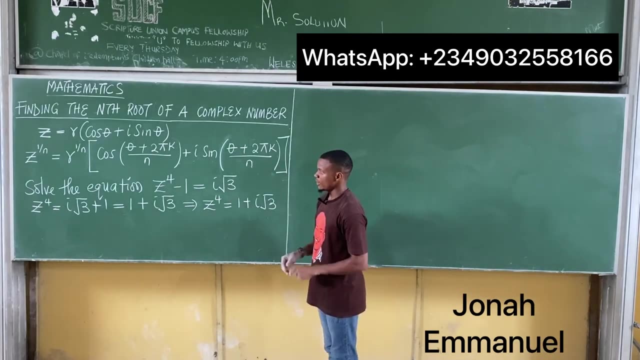 after my arrangement, it means that z to the power 4 is equal to 1 plus i root 3.. So I'm done rearranging the question Now. my question was to solve this, And to solve this means, of course, this is z to the power 4.. And perhaps I need to get the value of z And to get the value 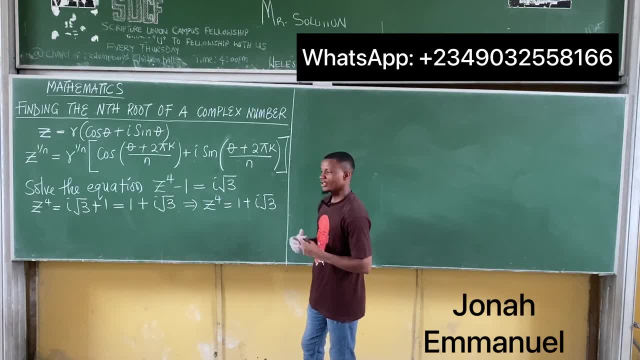 of z, I have to take the fourth root of both sides, of course. So I have to take fourth root. That means for this one here I'll have z to the power 4. multiplied by this is to the power 4,. 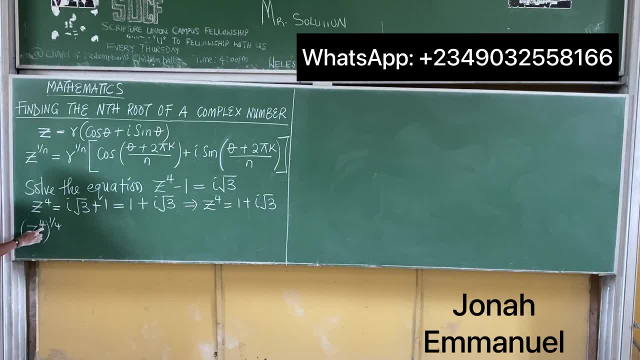 multiplied by 1 over 4.. This is the same thing as taking the fourth root. It's equal to my complex number 1 plus root 3i, root 3i, all to the power 1 over 4.. So I have this. So this, of course. 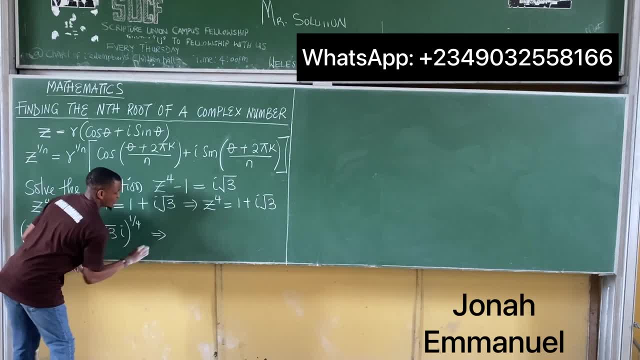 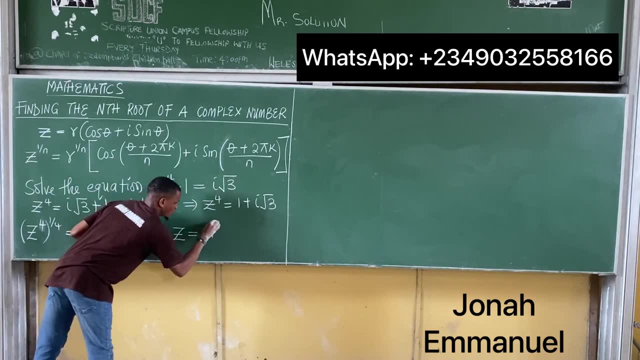 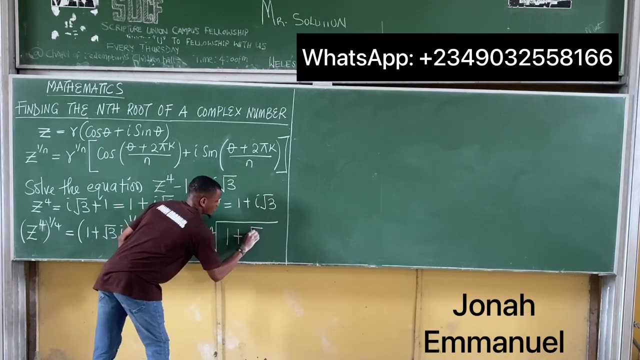 4 times 1 over 4 would now give me 1.. So I'll have this, So I'll have this, So I'll have this. So that would be equal to the fourth root of 1 plus root 3i. So I have this All right. So 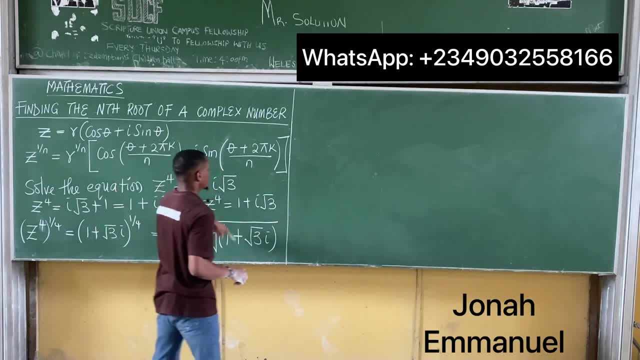 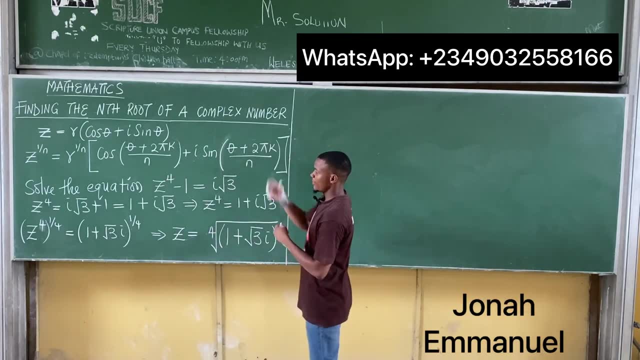 that's how we get z, So hence I'm looking for the fourth root of this. So in this case, to get the nth root, we need the value of n, And n is simply the root I'm looking for. 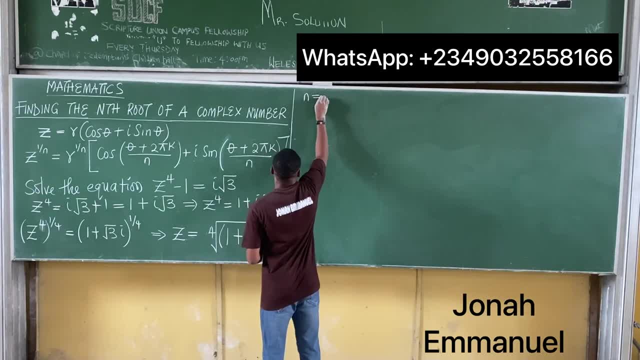 which in this case is the fourth root. So we can say n is equal to 4.. Next up, let's get r, the modulus. We said r would be equal to the square root of this one. here This is 1 squared plus this one. here This is root 3. 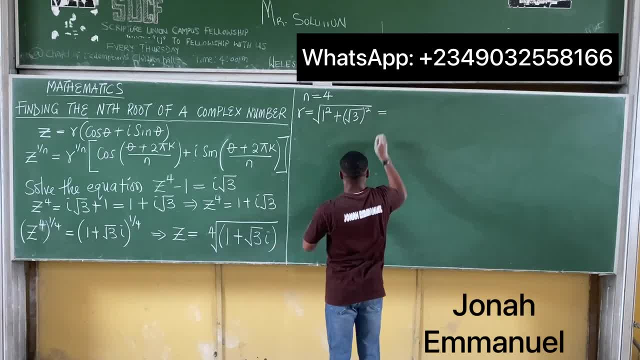 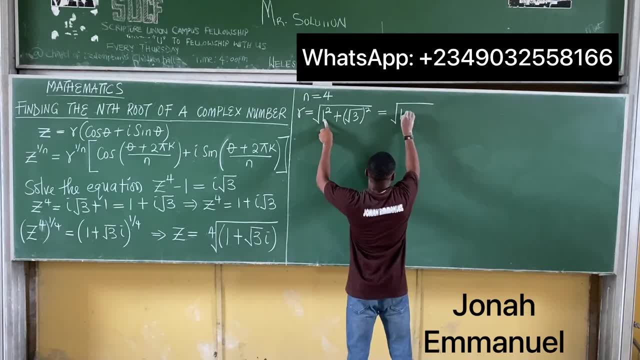 all squared, So that would be equal to. that would be equal to the square root of 1. squared is 1 plus root 3i, So that would be equal to the square root of 1. squared is 1 plus root 3i. 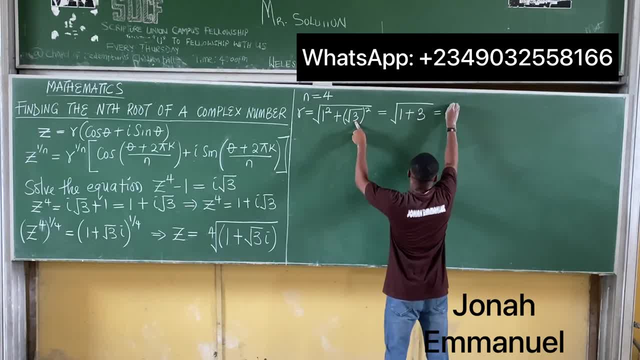 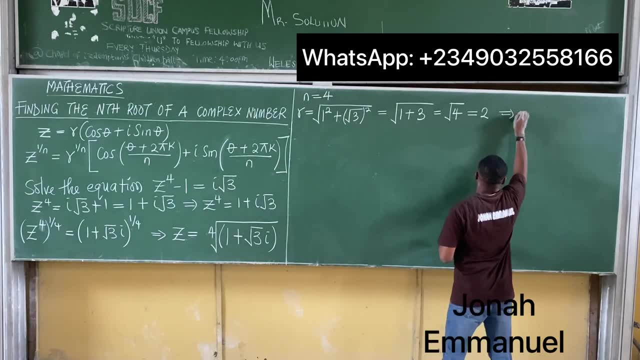 Root 3 all squared will give you 3., And that's equal to the square root of 1 plus 3 is 4.. Root 4 is equal to 2.. So that means that r is equal to 2.. Our next task is to find the value. 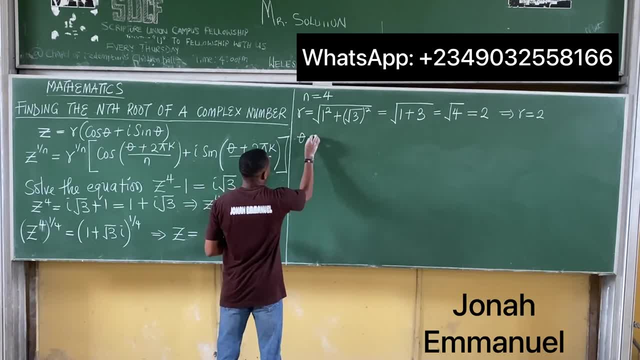 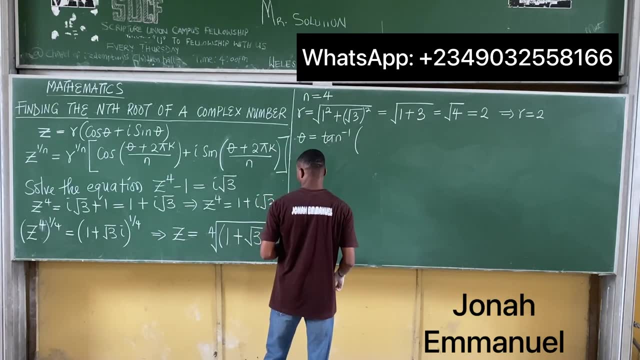 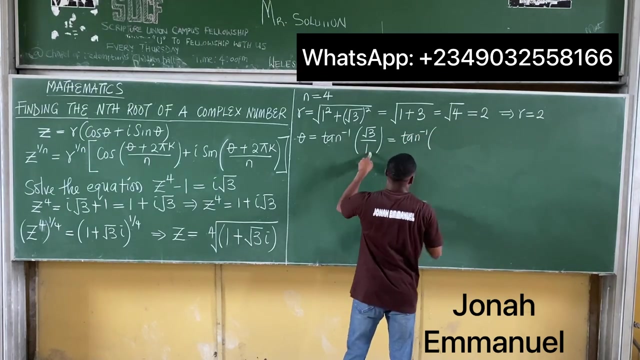 of the amplitude or the argument which is theta. We said it's equal to tan inverse of b over a. b here is root 3.. So it becomes root 3.. So I'm having 1.. So this is equal to tan inverse of root. 3 over 1 is root 3.. And if 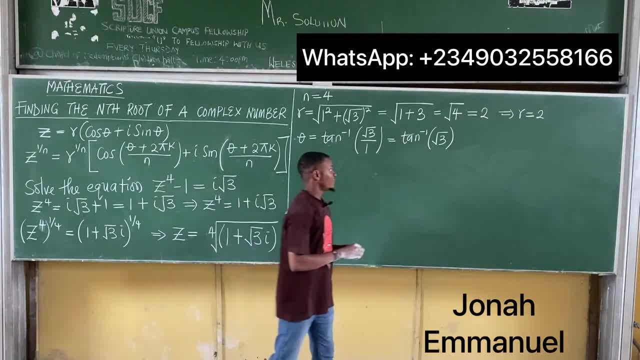 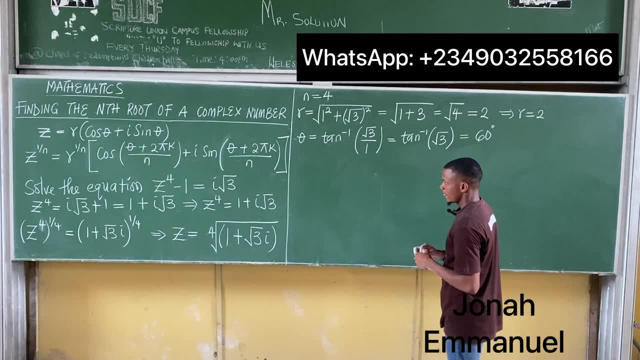 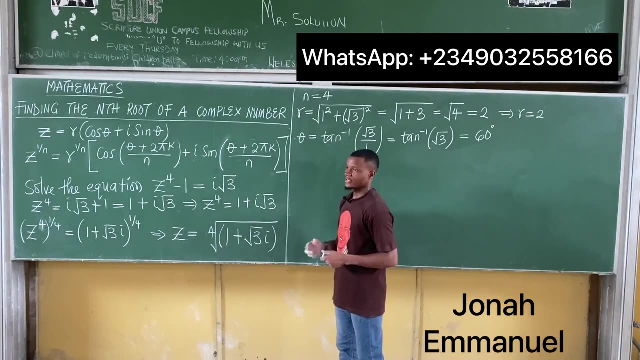 I get tan inverse of root 3, tan inverse of root 3 is equal to 60 degrees. So I'm having this as 60 degrees. So if I look at this one here, this is positive x and positive i. So since the two of these are in the first quadrant, we said in the first quadrant we 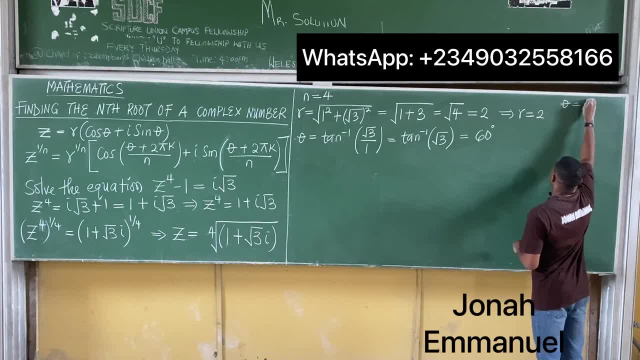 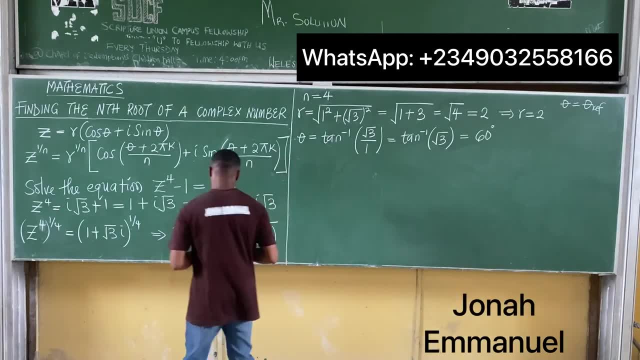 said in the first quadrant that my theta is equal to theta reference. We mentioned this in our last class, So hence there's no problem with finding the real angle. They're the same thing, All right? If that's the case, we can now go ahead and pull the answers, But for 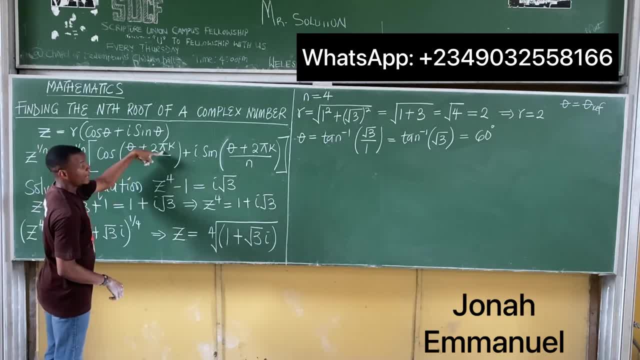 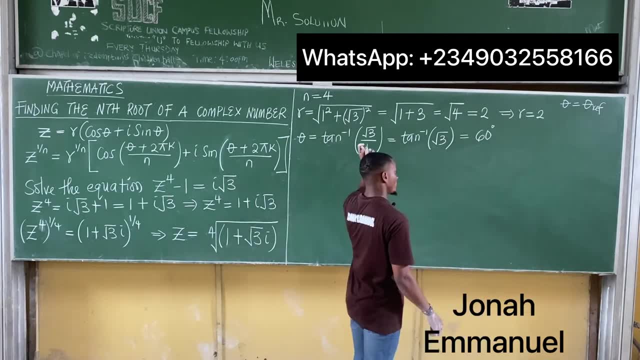 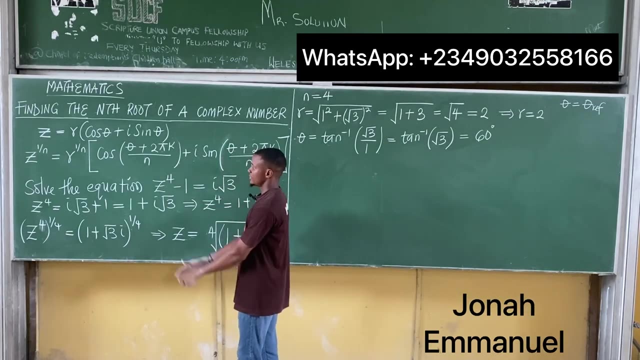 the fact that this one here is in what is called pi, that's in radians. we can choose to first of all convert this one here to radians first before imputing, Or invariably we can choose to put 180 here And put the answer in terms of theta. So it depends on which one we choose to. But 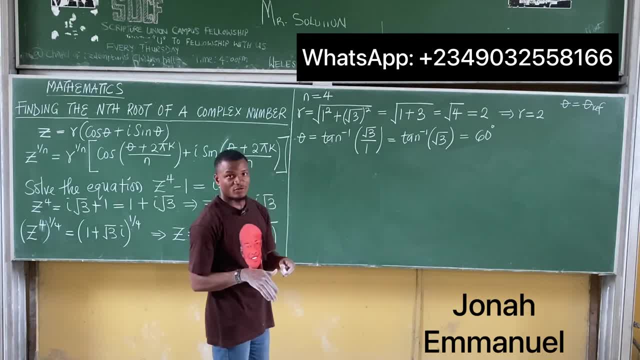 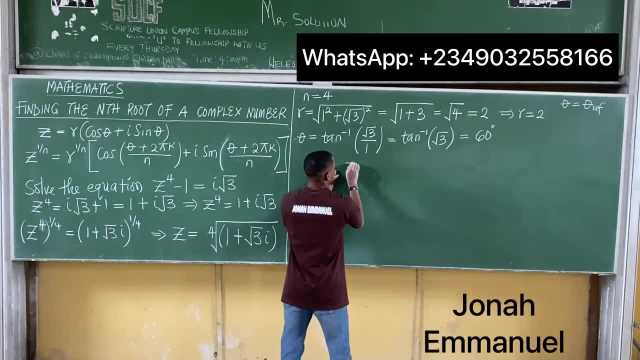 let's work with pi for this example. Let's work with pi first and then we'll convert to theta. So we work with pi, Converting this one here to pi. we said it's equal to to convert from theta to pi. multiply by pi all over 180.. From here this will cancel. 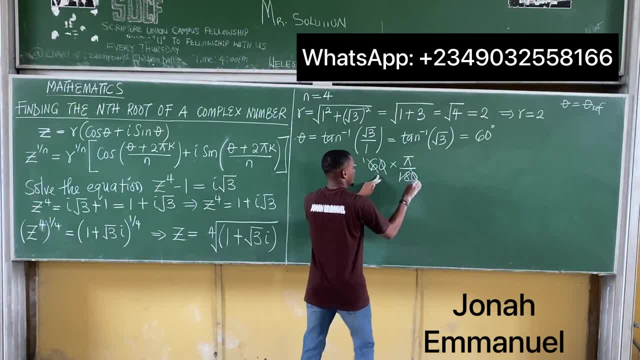 this: 6 here 1.. 6 here 3.. So this is equal to 180.. So pi over 3.. That's the value for theta, pi over 3.. All right, So if we've gotten this, 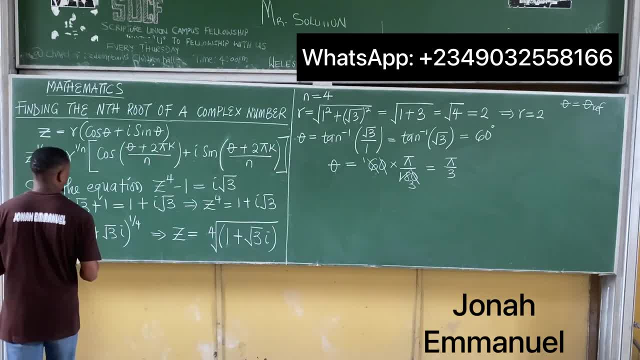 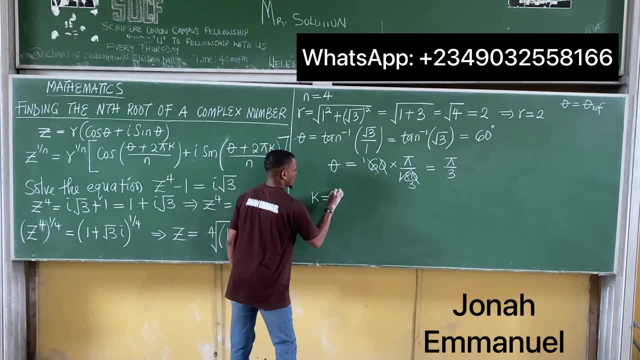 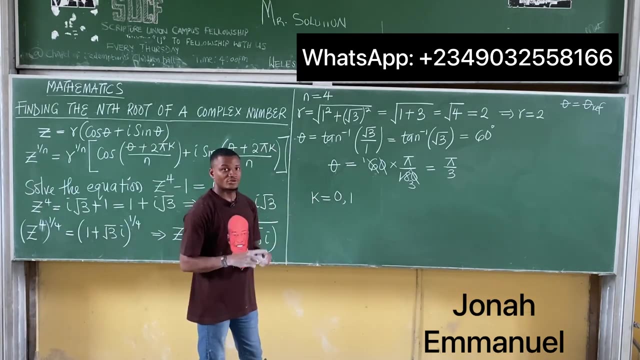 now. let's now get our fourth root. Now, this is how this works. To get your fourth root, first of all, put k as being equal to 0. This value gives you your first root. Then put k as 1.. This gives you your second root. Put k as 2.. This gives you your third root, And 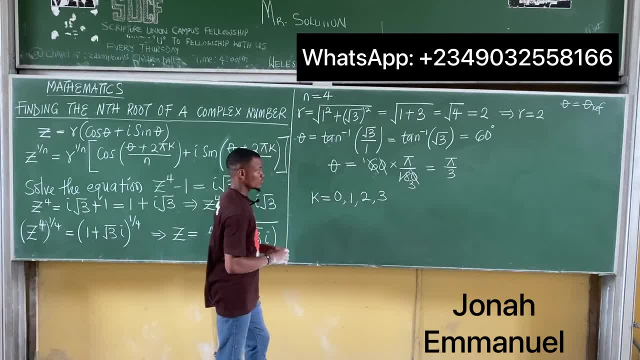 then put k as 3.. This gives you your third root, And then put k as 3.. This gives you your fourth root. If I still want to get the fourth root, I'll simply put k as what there? 3.. Please, this is how this works, Alright. 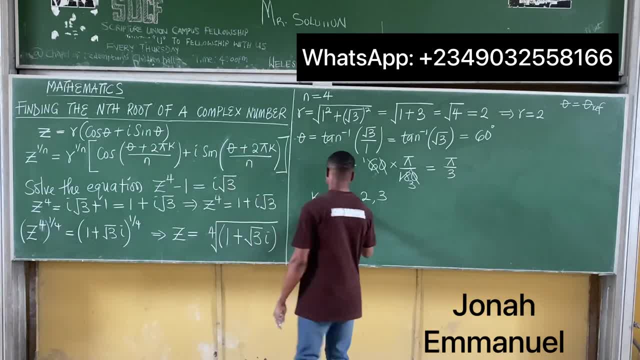 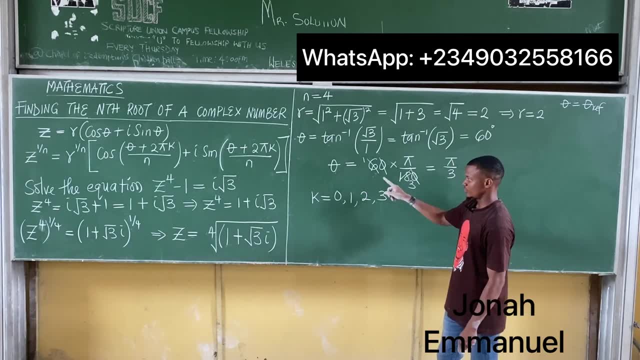 If you say: find the first root. the first root is k equal to 0. Second root, k is equal to 1.. Third root, k is equal to 2. Then fourth root, k is equal to 3.. Alright so. 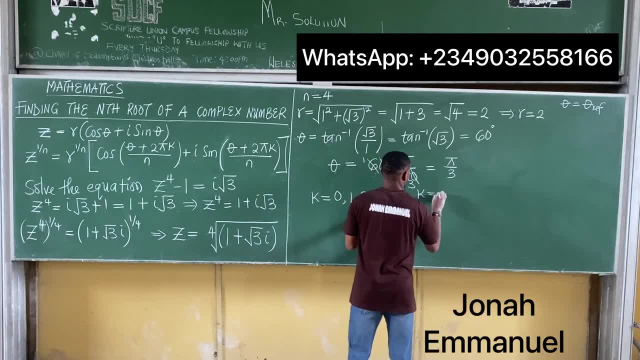 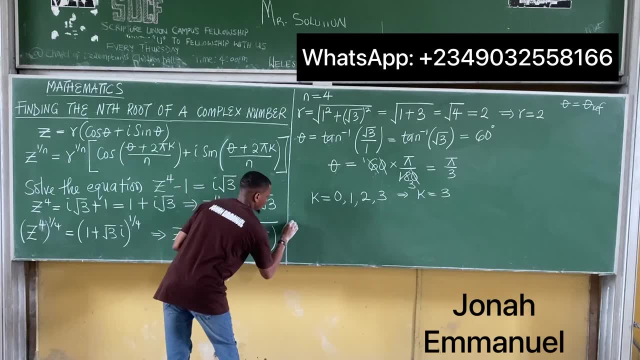 in this case, fourth root, it means that k is equal to 3.. Alright, so if we replace this, if we replace this, so it means that z to power 1 over n is 4.. 4 will be equal to. they said r to power 1 over 4.. What's r here? 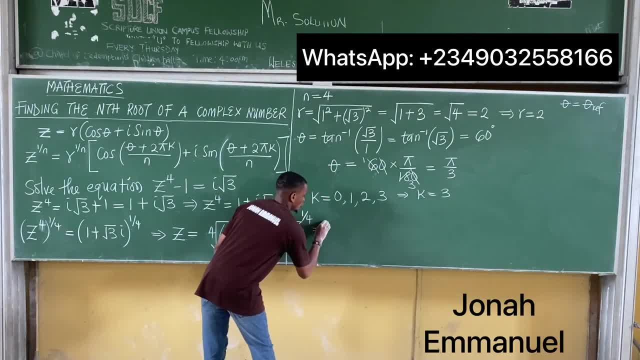 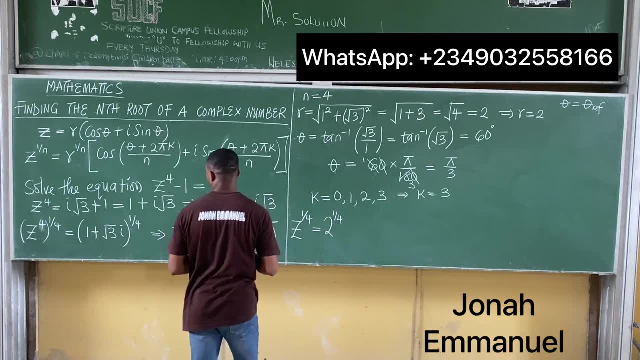 r is 2, so it becomes 2 to power, 1 over n, 1 over 4.. So 2 to power 1 over 4 into cos. so this is into cos 2.. Theta in terms of pi is pi over 3.. 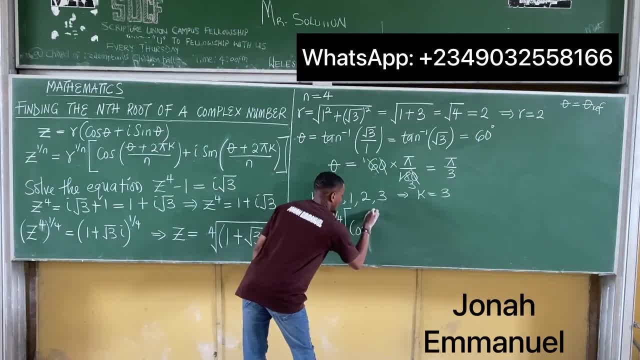 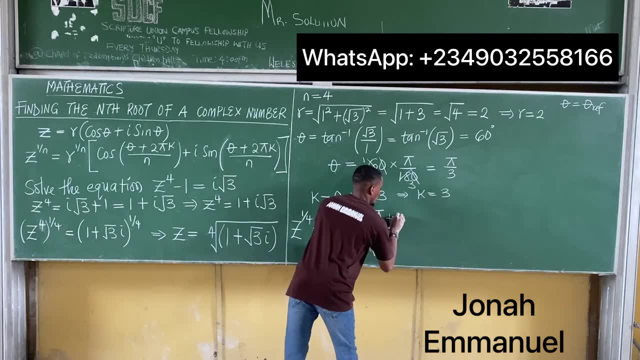 So I'm having- okay, I'm having this as cos: pi over 3 plus 2 times pi times k, k is what there 3.. So 3 for fourth root all over n, n is what there 4.. So I have this. 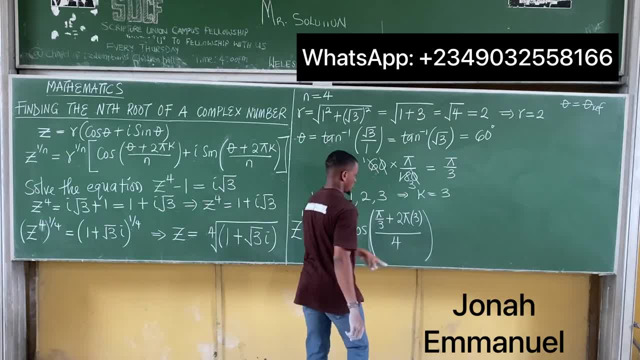 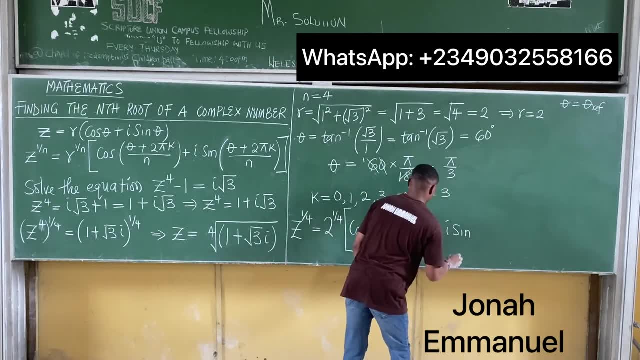 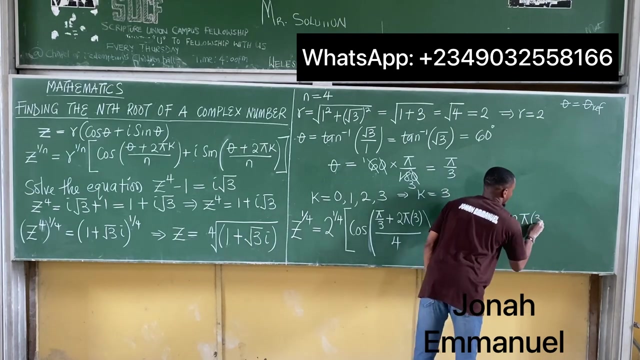 It becomes this one here. But no problems, Plus, so plus i sine theta, which is pi over 3.. So pi over 3 plus 2 pi k. for the fourth root we say k is 3, all over n, n is 4.. 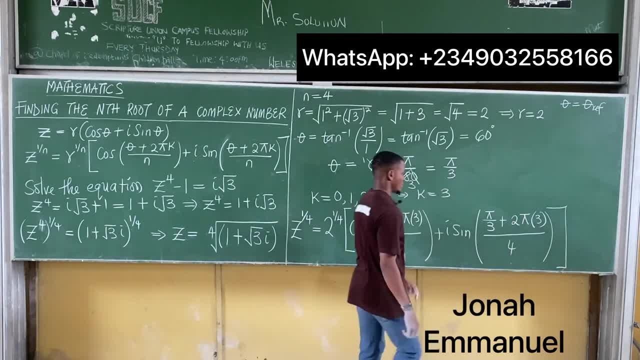 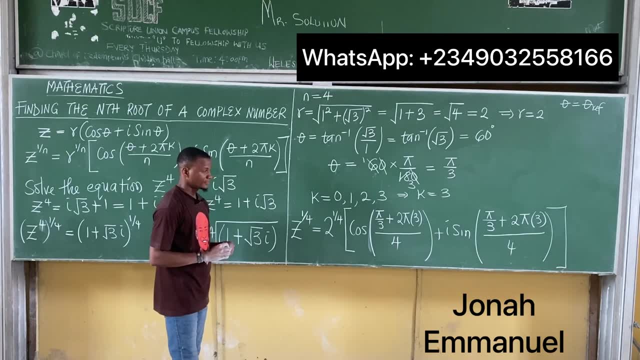 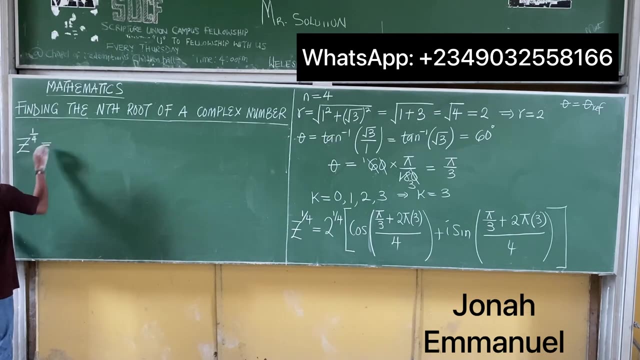 Fourth root. I have this, So if I can simplify this, it gives me the fourth root of this complex number. All right, So to simplify this, I'll be having: z to power 1 over 4 is equal to 2 to power 1 over 4. 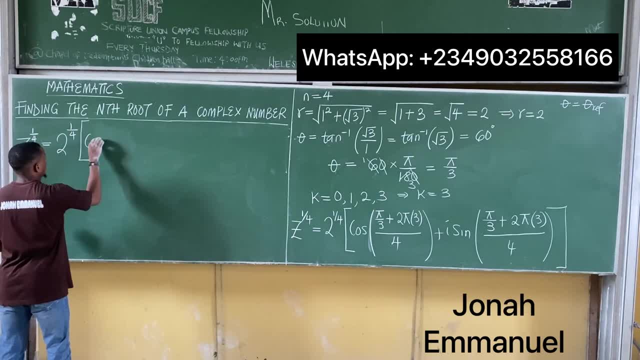 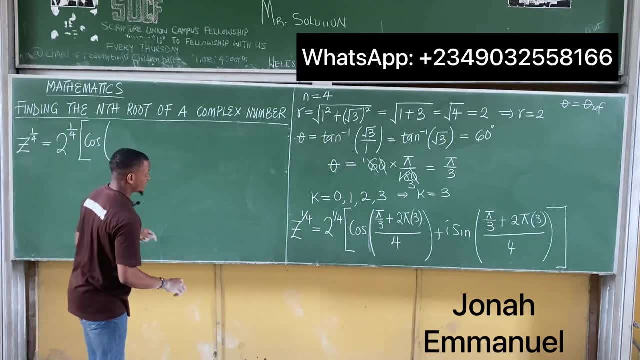 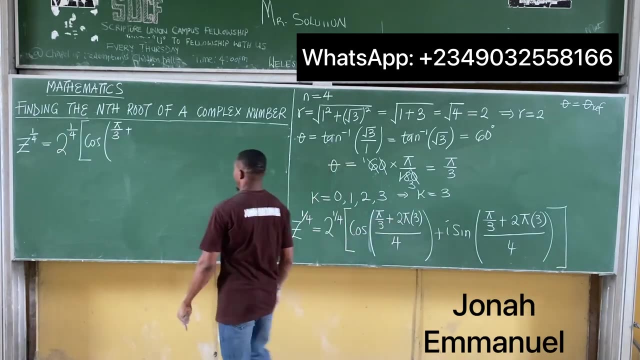 into cos, that's cos of work with the numerator. With numerator I have pi over 3, that's pi All over 3.. Plus this gives you 2 times 3. That's 6 pi. So plus 6 pi. 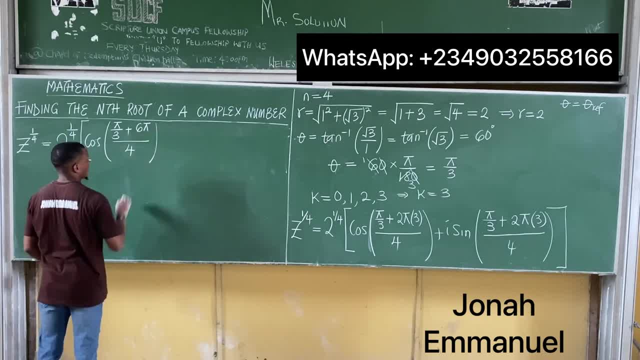 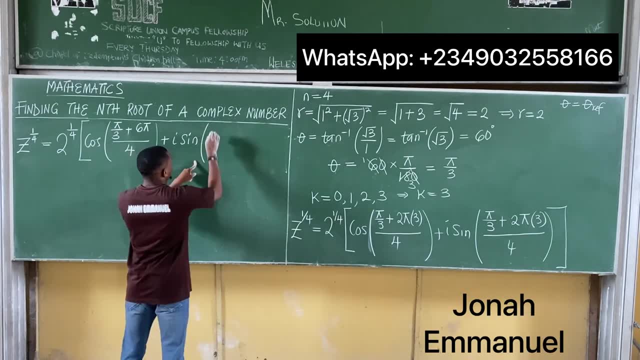 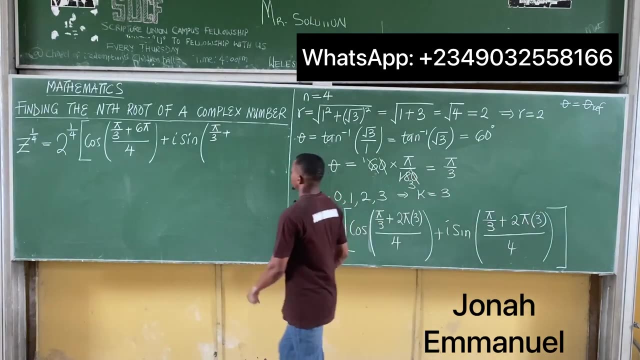 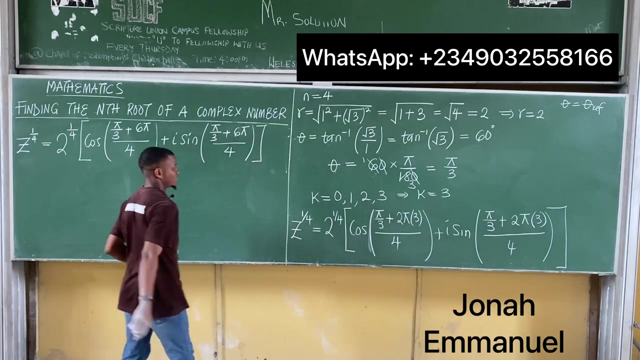 all over 4. 4.. I have this Plus i sine same thing there. root 3 pi over 3 plus 2 times 3 times pi is 6 pi. So plus 6 pi all over 5.. 4, we have this. alright, simplifying for now. what do we get? we have this z to the 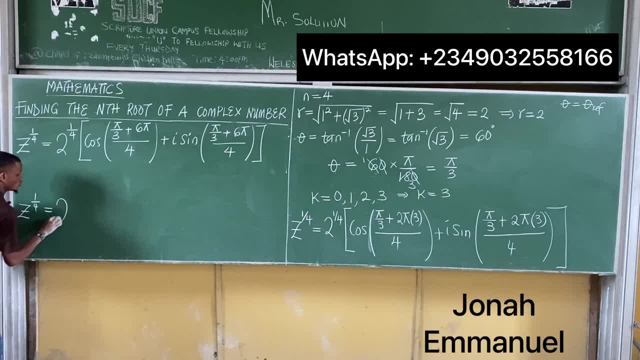 power 1 over 4 is equal to 2 to the power 1 over 4, into we have this to be cos, so cosine of numerator, my LCM here is 3, so I'm having 3 into 3 by 3, 3 divided by 3 is: 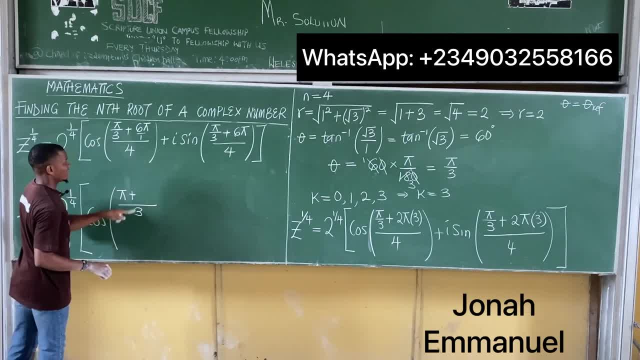 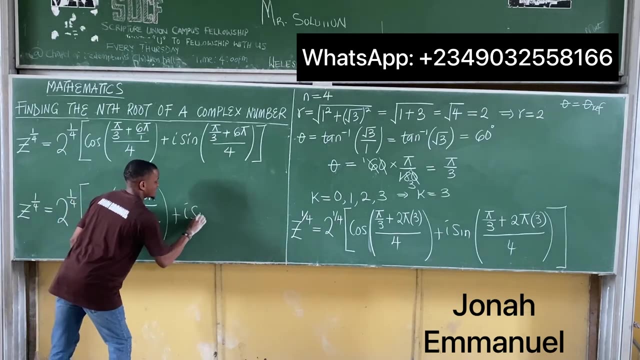 1, times pi is pi plus 3. divided by 1 is 3, times 6. pi is 18 pi. so I have this all over 4, so this is numerator all over 4, plus pi sine. so these are the same thing. 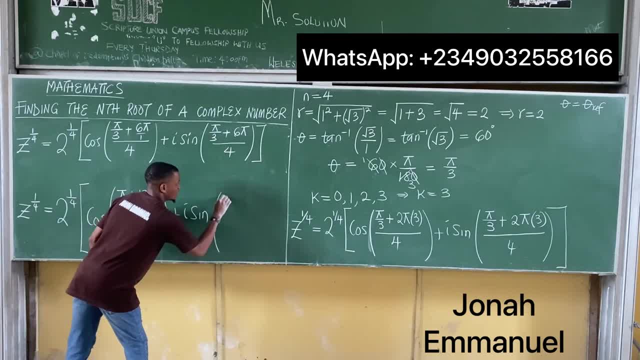 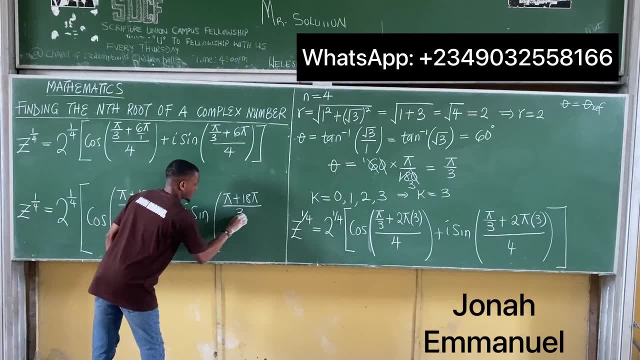 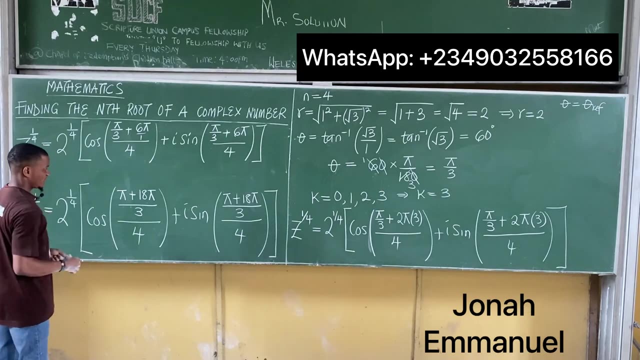 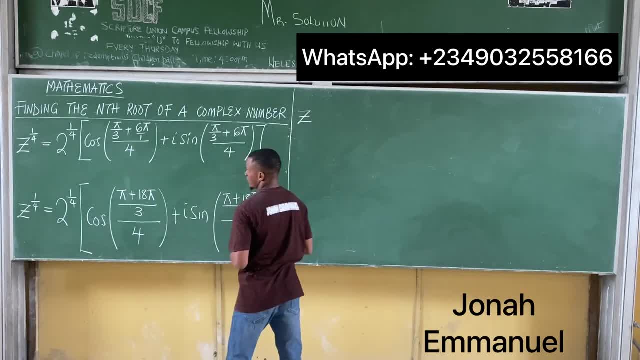 it means that the 4 to the power 1 over 4 is equal to 2 to the power 1 over 4, so this is so. that's z is please, not z to the power 1 over 4, but just z, please, just z. 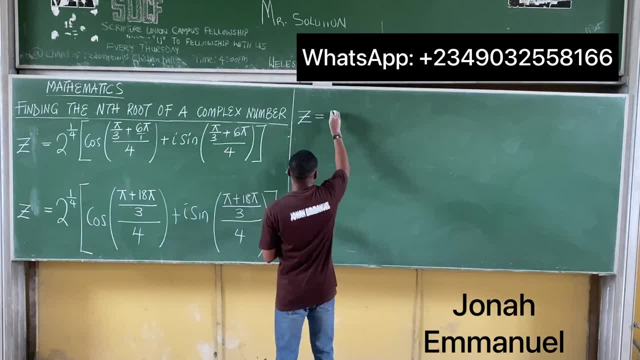 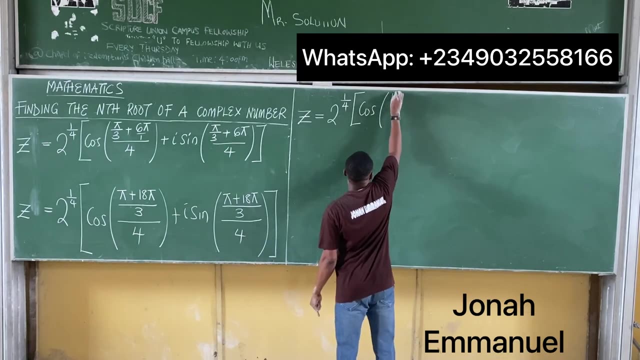 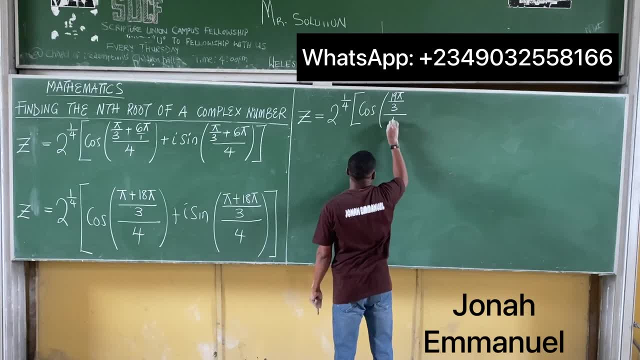 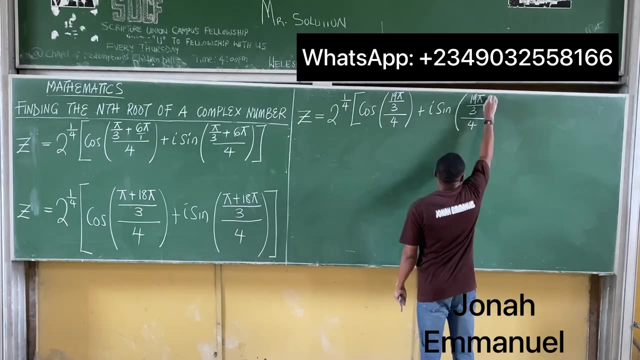 19 pi all over 3,, all over 4, I have this plus i sine same thing here: pi plus 18 pi gives you 19 pi. so 19 pi all over 3,, all over 4, we have this one here, alright, let's. 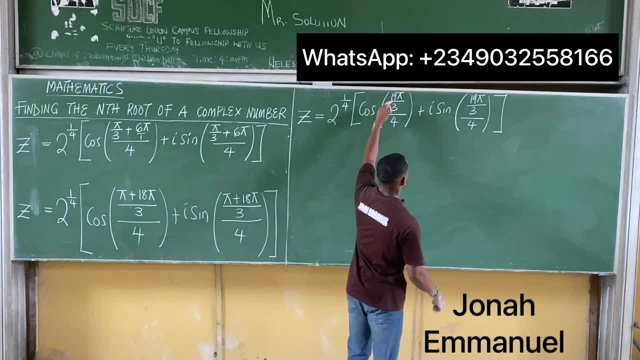 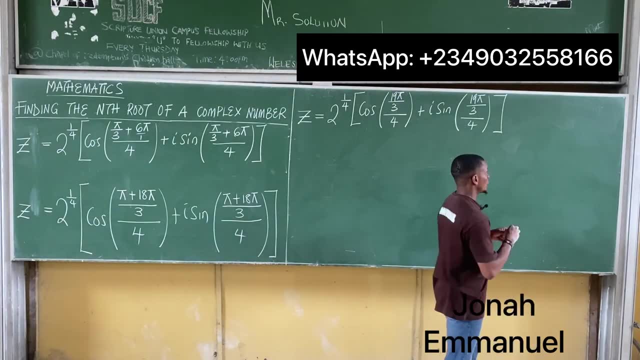 proceed? how do we simplify a fraction like this? what do we do? the idea is simple. if I have a fractional numerator or all over a denominator, let's say in the form a over b divided by c, this can still be written as a over b divided by c, and that would be a over. 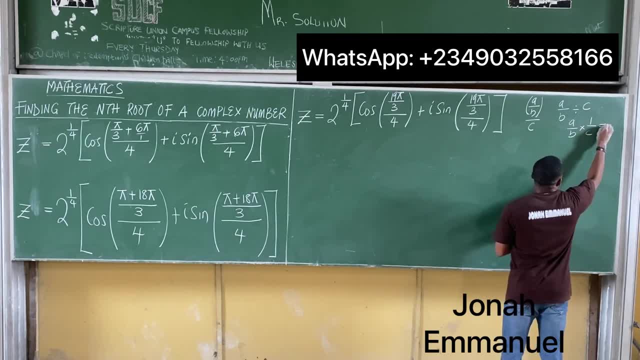 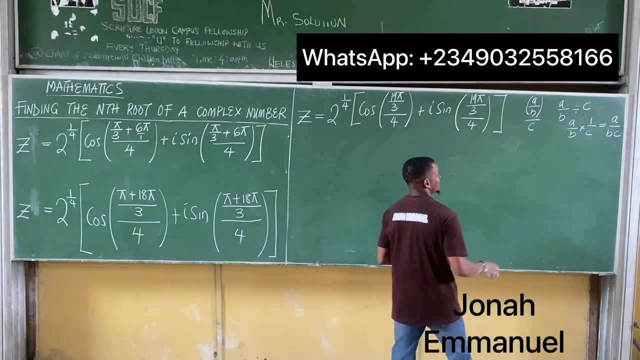 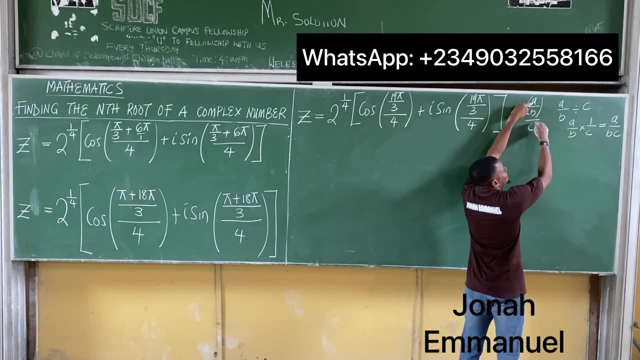 b times. invert this 1 over c. that's equal to a all over b times c is bc. so the concept is simple for cases like this, simply hold on to numerator and multiply these two so a all over b times c. so if that's true, that means z is equal. 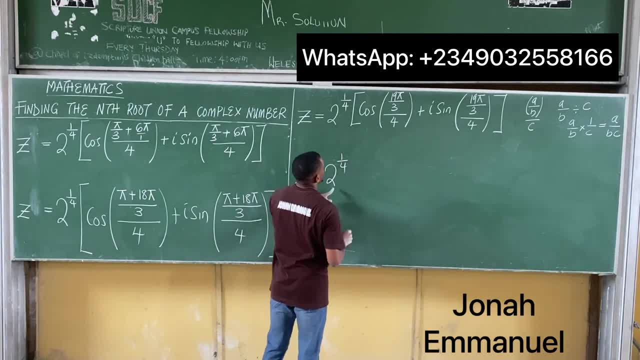 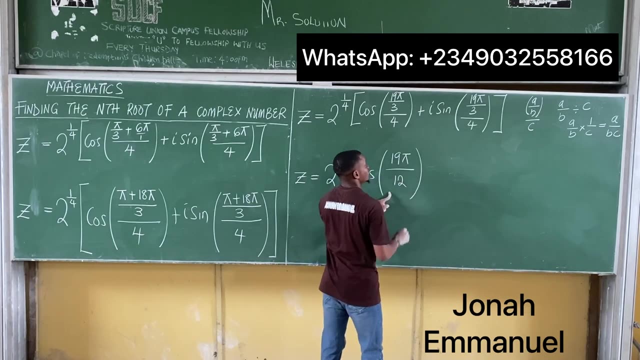 to 2, to the power 1 over 4, into. I'm having this as cos we said. hold on to numerator, that's 19 pi. multiply these two 3 times 4,, that's 12,. I have this plus i sine. 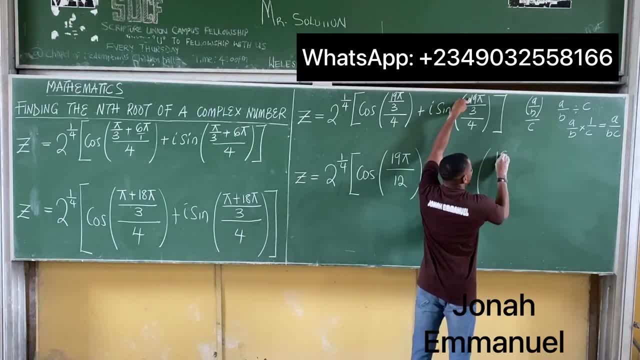 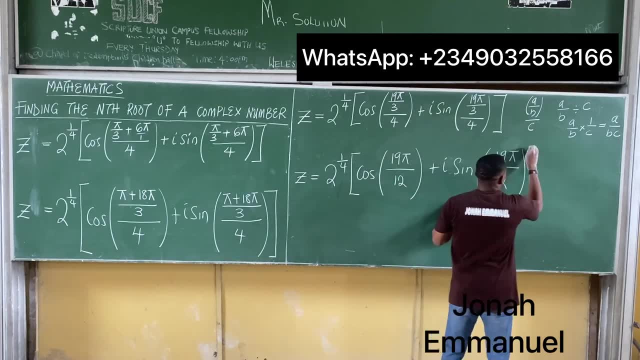 here. hold on to numerator, that's 19 pi all over. multiply these two 3 times 4,, that's 12, so I have this alright. so I think this is our answer right. so this is how we get. 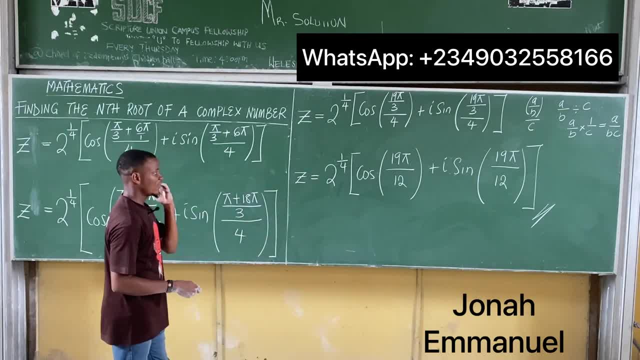 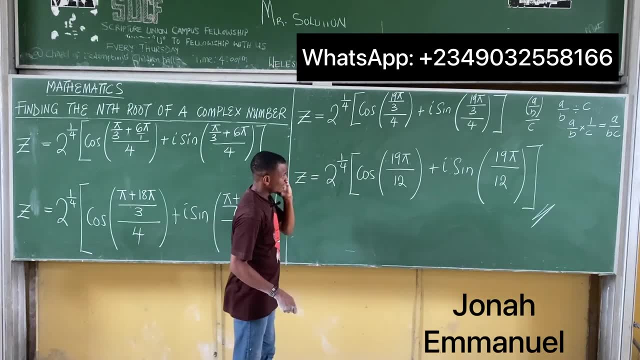 this, this becomes the fourth root of that complex number. so this is how we solve this. we can choose to present our answer in what is it called. we can choose to present our answer in rectangular form. and how do you do that? first of all, convert this to polar form. so put pi as 180, simplify. 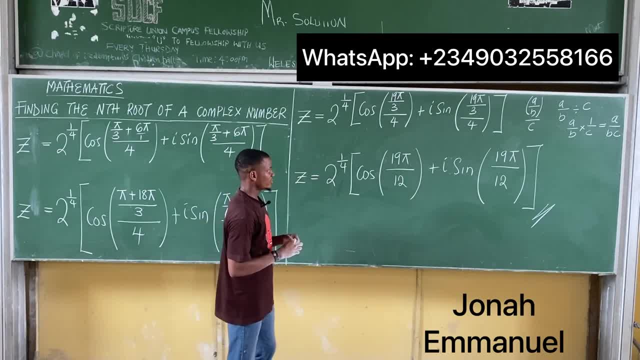 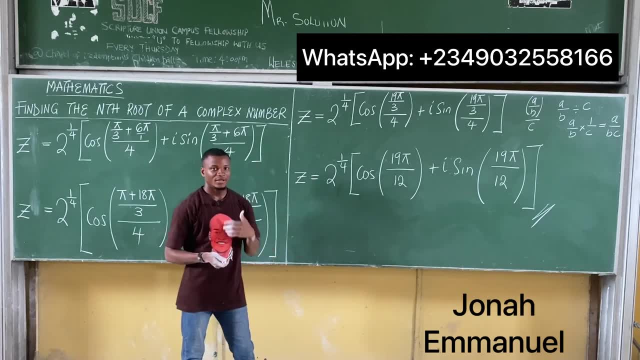 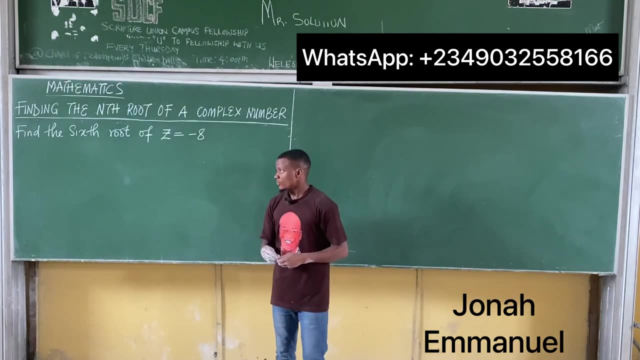 and get your final answer. or, invariably, you can choose to punch this directly in terms of radian and you get your final answer. so that's how you solve this question. alright, so we'll take this example on finding the nth root of the complex number. so we'll 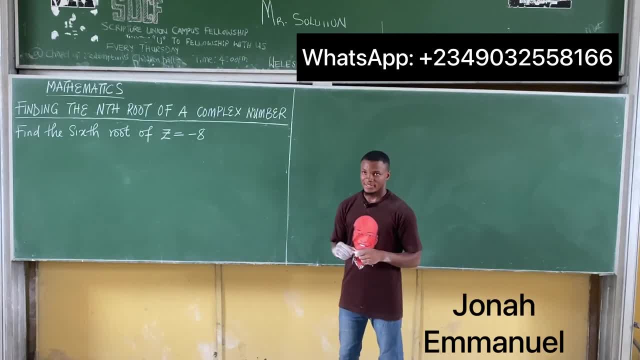 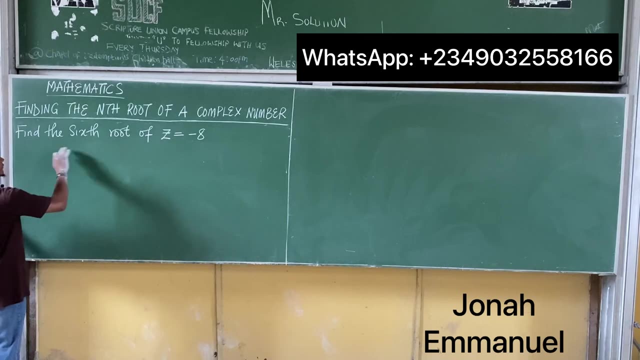 see this in this question. we're we're given that z is equal to minus 8, and we'll actually find the sixth root of this ofcourse. here's equation on complex numbers. how do we solve this? first things first, let's get the value of n. record that the formula for finding 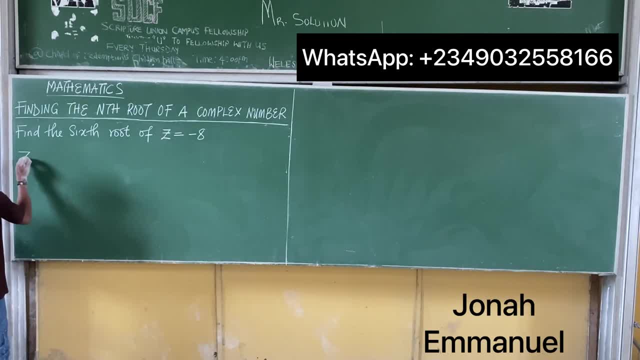 the nth root of the complex number is z to the power 1 over n is equal to r to the power 1 over n into cosine pi. Okay, so now we've seen that, since we're looking up to 앉 Då Dan Ayub, and now we're 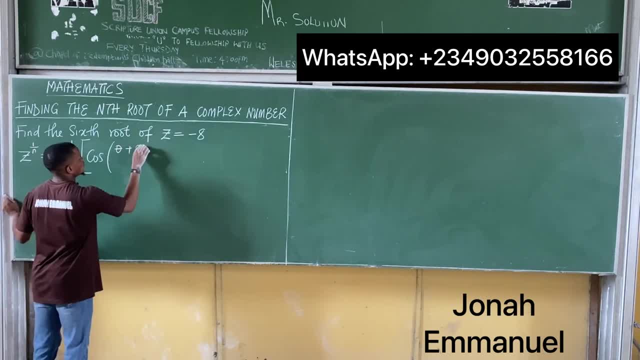 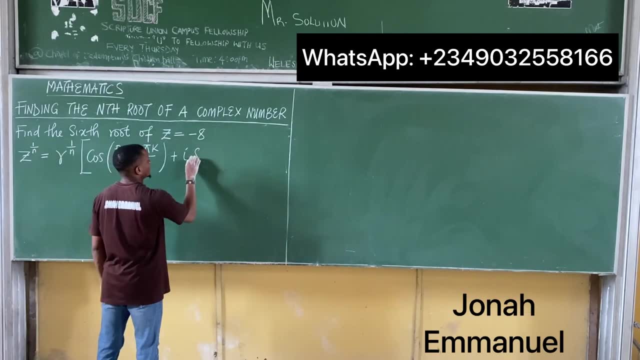 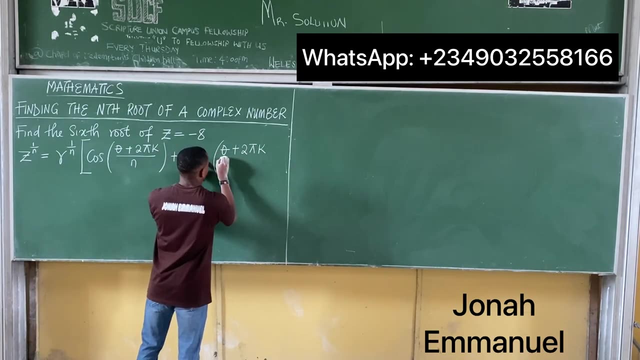 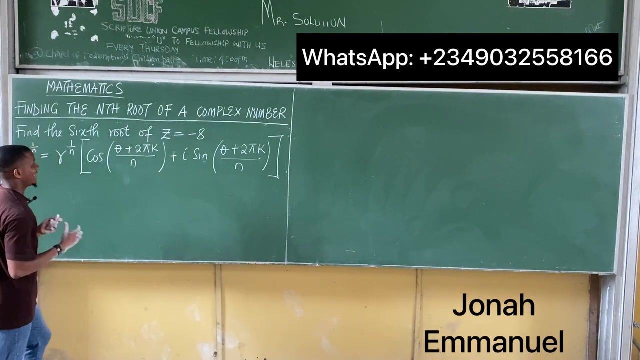 of theta plus 2 pi k all over n. this plus i sine theta plus 2 pi k all over n. we had this as the formula for finding the nth root of a complex number. all right, so how do we do this here? first is first: what's n? n is equal to the required root, which in this case is the sixth root. 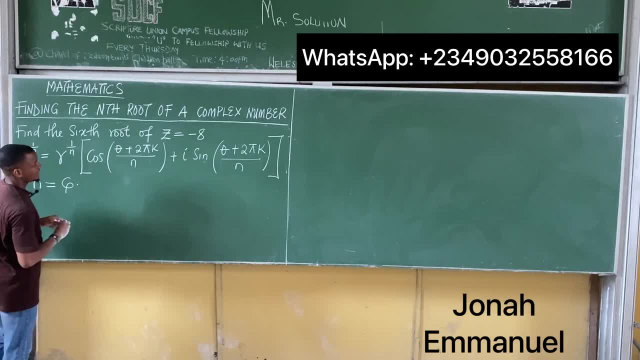 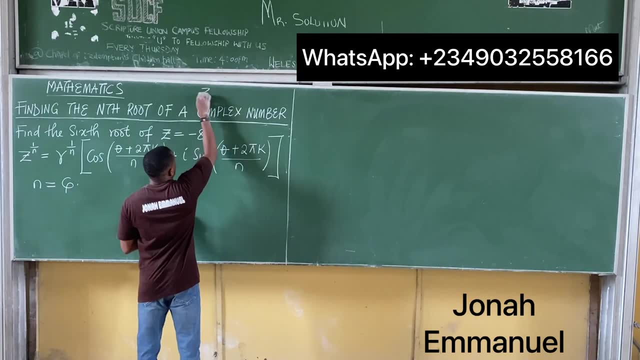 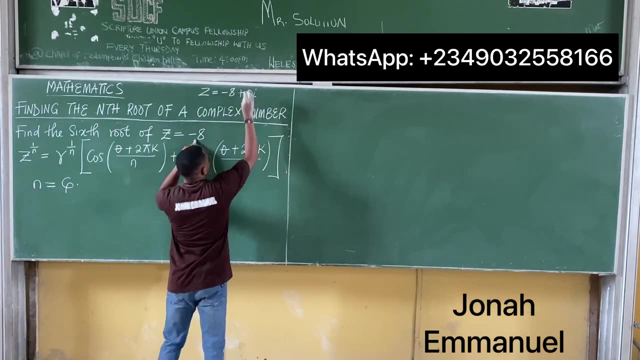 so i have n as six. next up, let's find the value of r, the modulus. we said in this case. so if i'm given that z, if i'm given that z is equal to minus eight, the full form of this would be minus eight plus zero i, as we discussed in our previous classes. so hence the value of r, the modulus. 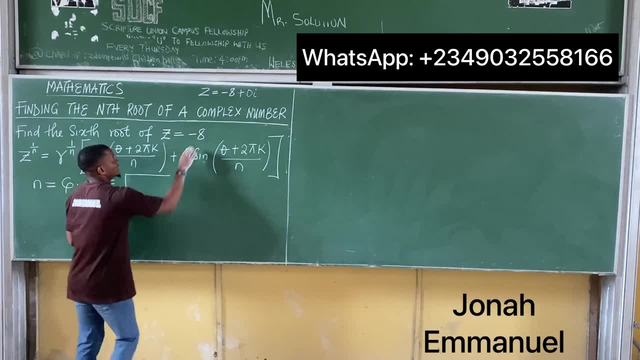 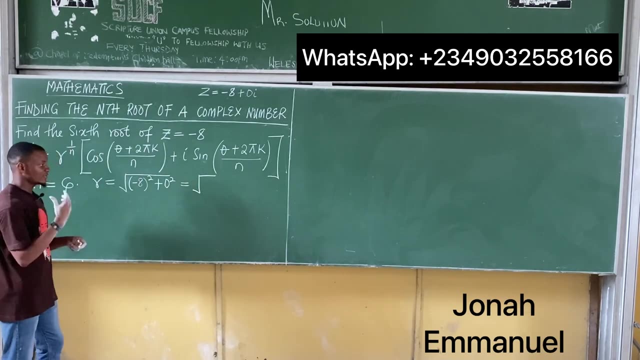 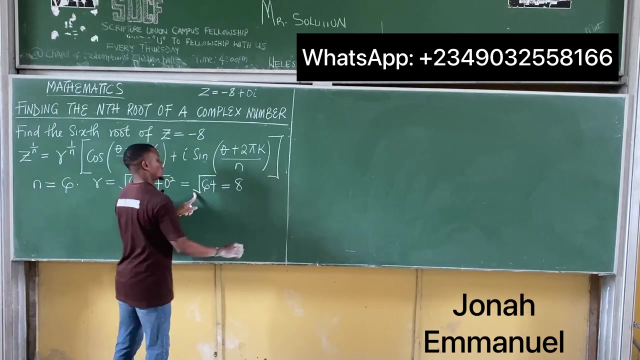 will be equal to this square root of this square, that's minus eight r squared plus zero squared- which this one does not matter, so i'll just focus on this- becomes the square root of minus eight. squared means minus eight times minus eight. that's equal to 64. so positive 64 root 64 is equal to eight. 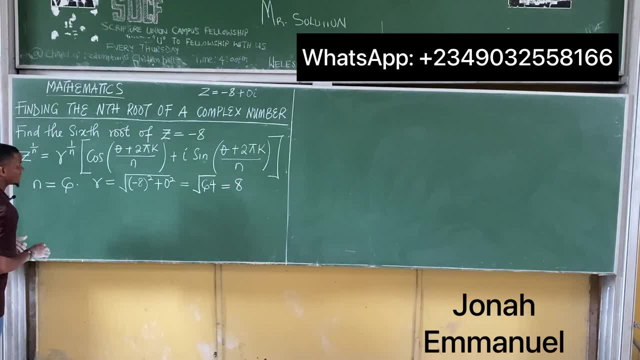 so the modulus is eight. let's get theta. now we said for cases of this one here to get theta, our best idea would be to draw the aghan diagram for this. in this case of minus eight and zero, my, uh, my coordinates would be minus eight for x and zero for i, so drawing minus eight. 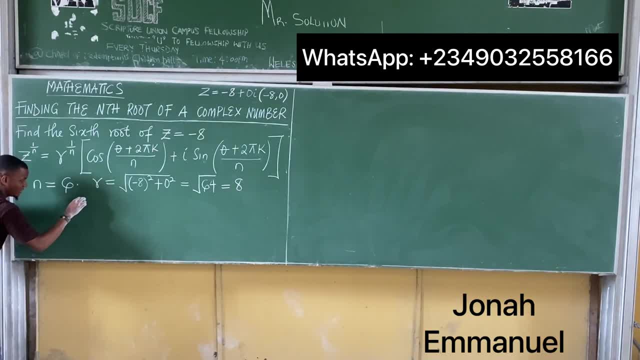 on the aghan's diagram becomes something of this nature here. so this and this, this is positive x, this is negative x, my, this is negative x minus eight will be somewhere here. so say, as minus eight, my angle becomes from here- we said from the positive x angle up to this point here- so this will become the angle which is 90 degrees. 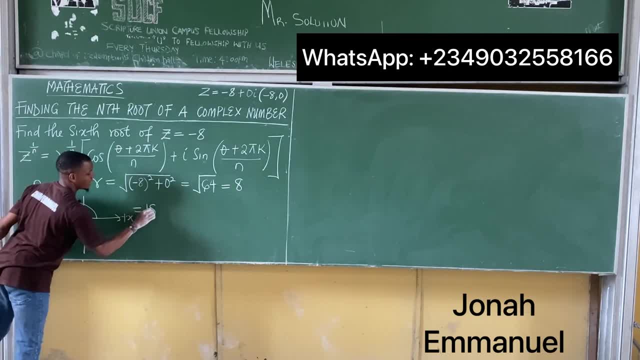 plus 90 degrees, that's equal to 180 degrees. so my, my angle here, or the argument, or the amplitude theta is equal to 180 degrees because it's negative of x minus eight and i have this, so it becomes this. we will explain this concept in our previous class, so if you've not watched the 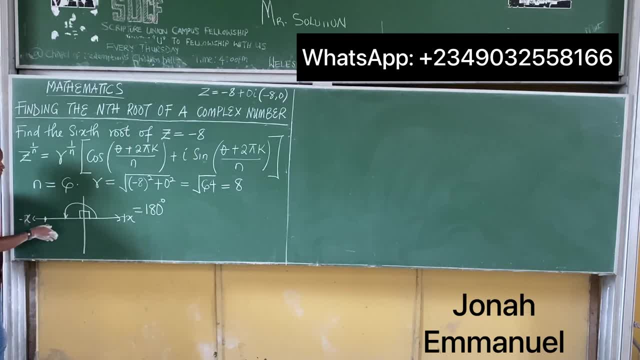 video on how we got this. i'll leave a link in the description of this video on how we got this value here. all right, let's proceed. i'm not forgetting that we've said theta, which is equal to 180 degrees, but then, uh, from our formula, here we're working with the radian value, so perhaps let's. 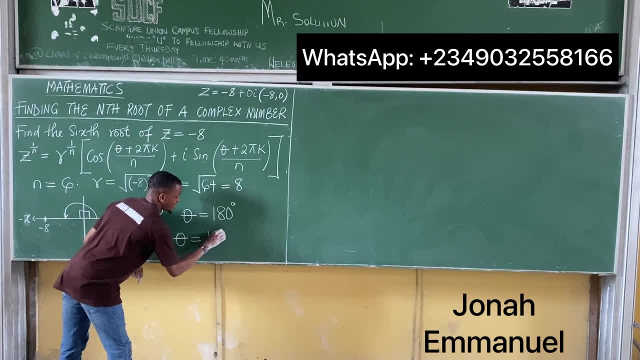 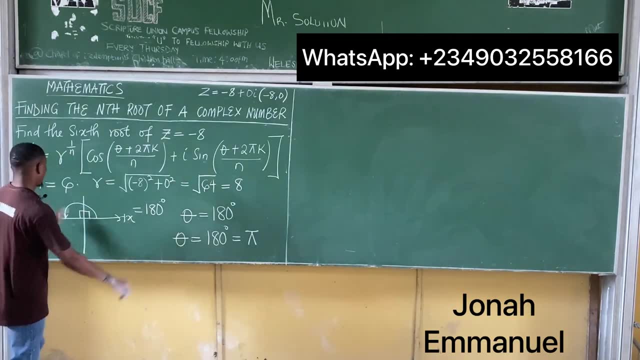 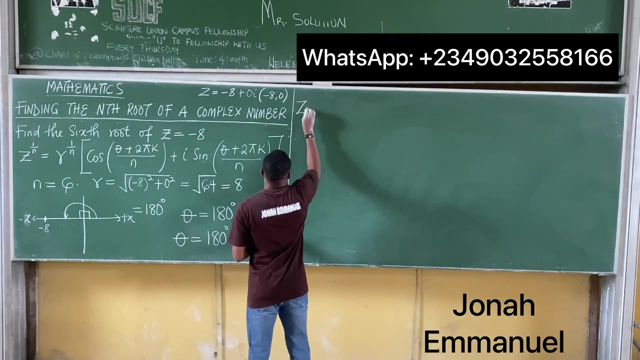 convert this to radians, 180 degrees, we said it's equal to what there one rad or one pi rad, so that's equal to that which is equal to one pi by six. so that means my answer is this: it means that the sixth root of this that means z to power, one over six, that's six roots, which is equal. 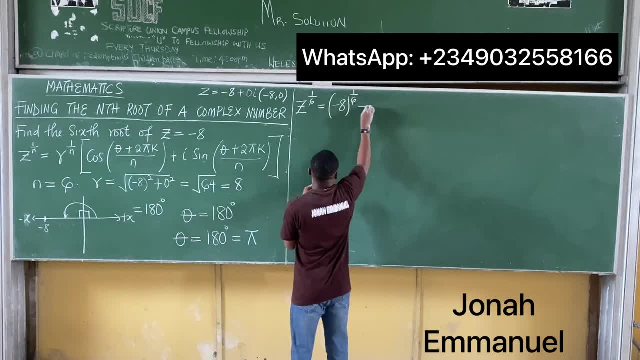 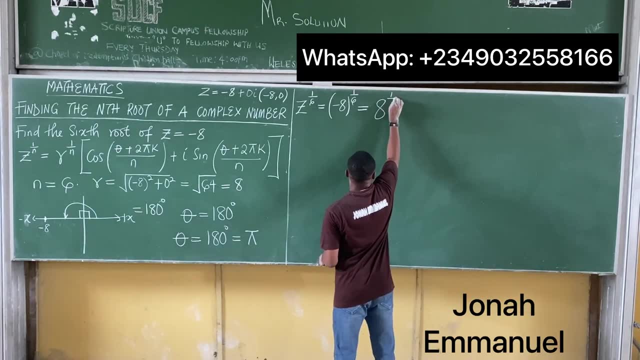 to the sixth root of minus eight, the sixth root of minus eight will be equal to first. since first r r is eight, it becomes eight to power one over six. sixth root of the of the modulus multiplied by so does this into cosine, so cosine of theta, theta here, in terms of pi. in terms of pi. 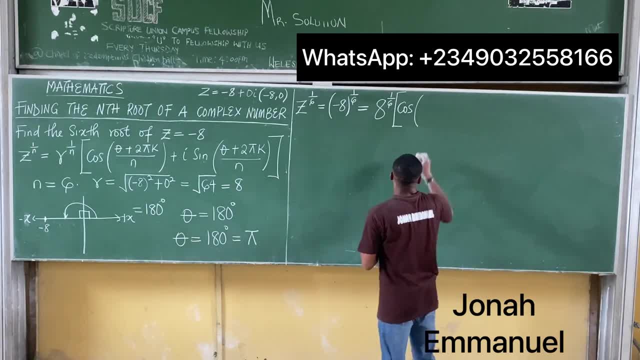 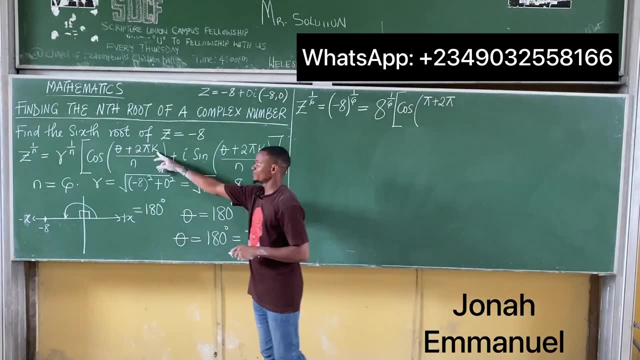 is pi, that's 180 degrees, which is pi, so it becomes pi, no longer theta plus 2 pi. okay, so we are yet to get k. Let's get k. what's k? We said? the idea is simple, that. 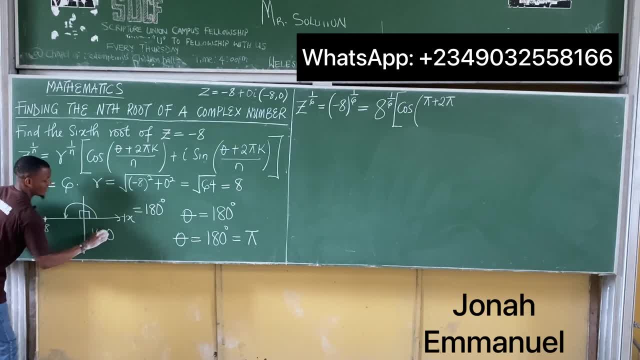 k starts from 0, so we have: k is equal to 0, this becomes the first root. for second root, k is 1,. for third root, k is 2,. for fourth root, k is 3,. for fifth root, k is: 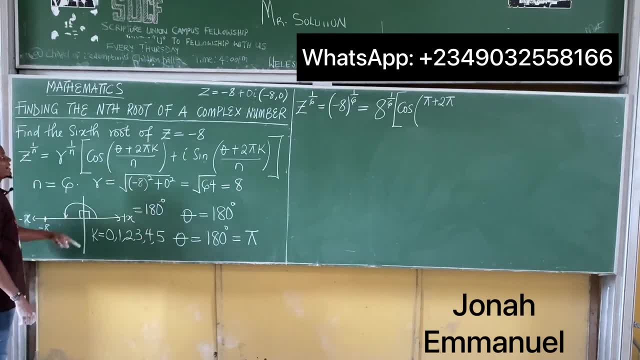 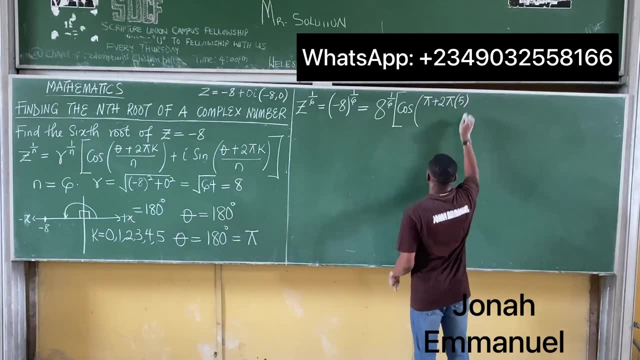 4, for sixth root k is 5.. Since I'm actually finding sixth root k becomes 5, so I have this as this into: k becomes 5, that's for the sixth root all over n. n is 6.. So I have. 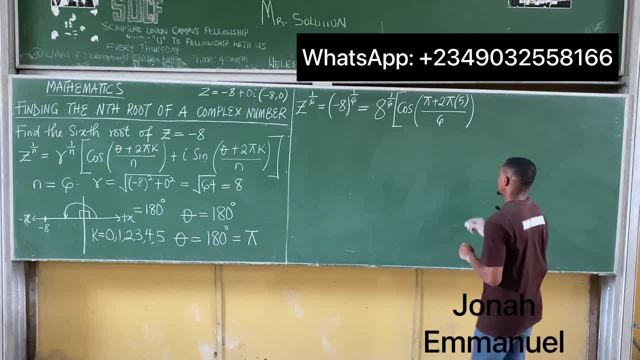 this one here, plus i sine. next up I have theta. theta is pi, that's 180 degrees plus 2 times pi, times k. we said for sixth root, k is 5, so it becomes times 5, all over 6,. 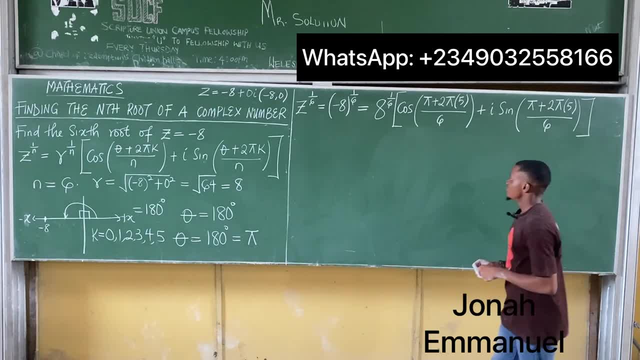 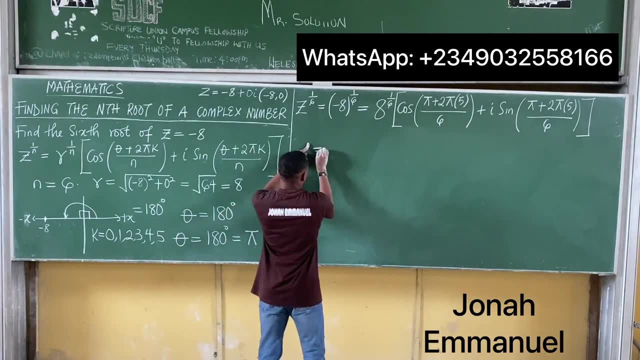 so I have this case here, alright. So this is what I have. alright, simplifying this one further, what have we got? This would be equal to this, would be equal to h, to the power 1 over 6, okay, into this. 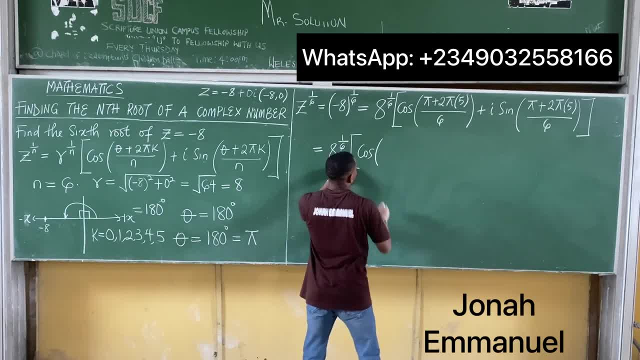 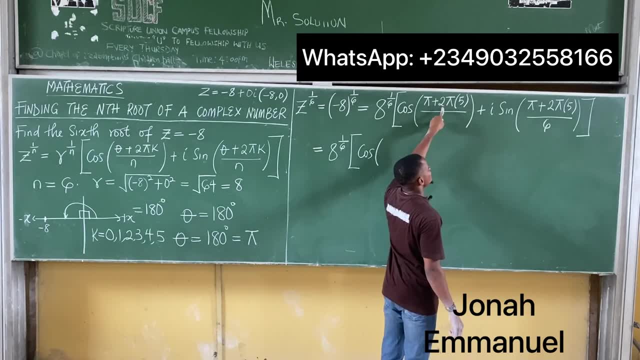 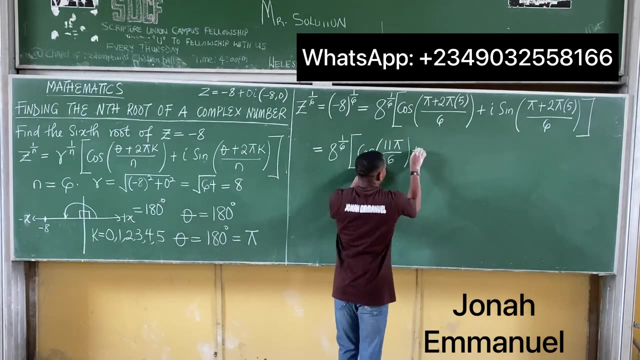 is into cosine of. this is 2 times 5, that's 10 times pi, that's 10 pi. so pi plus 10 pi gives you 11 pi. that gives you 11 pi all over 6, plus i sine. 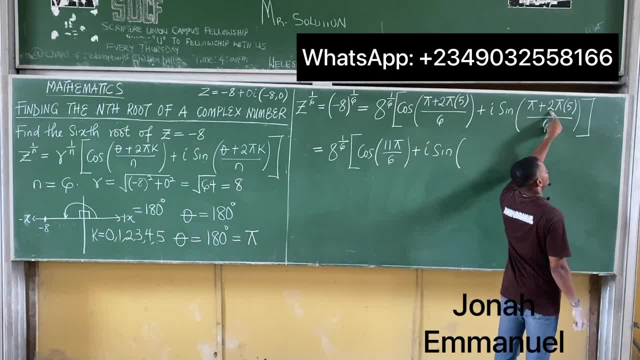 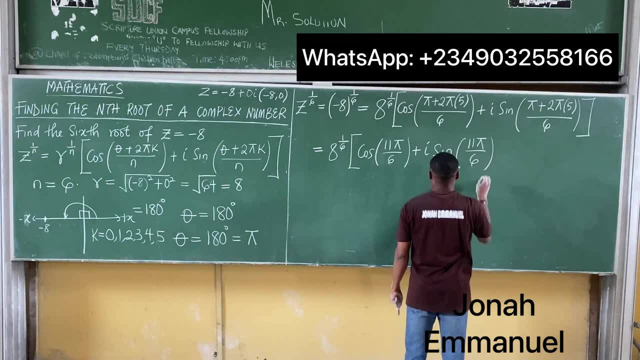 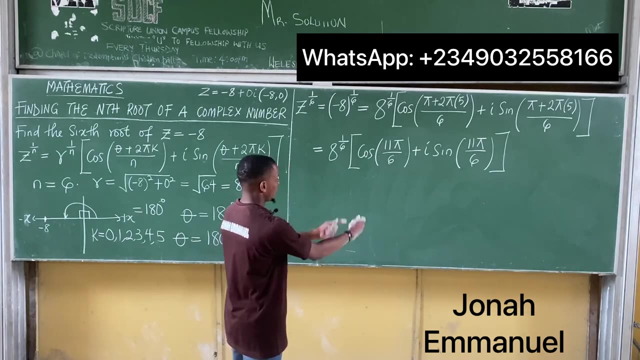 Same thing here 2 times 5 is 10 times pi. that's 10 pi plus pi. that gives you 11 pi. so this is 11 pi all over 6, so I have this work here. Alright, so this is probably our answer. this is our answer. okay, we can choose to if 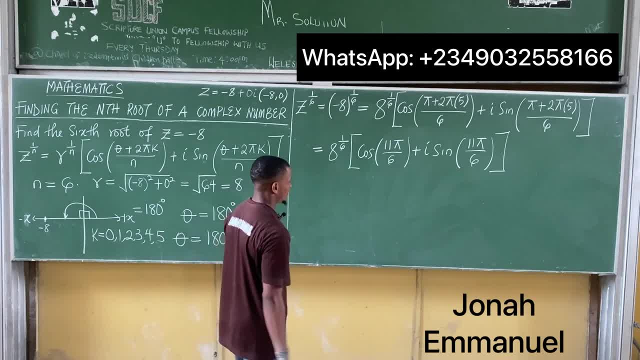 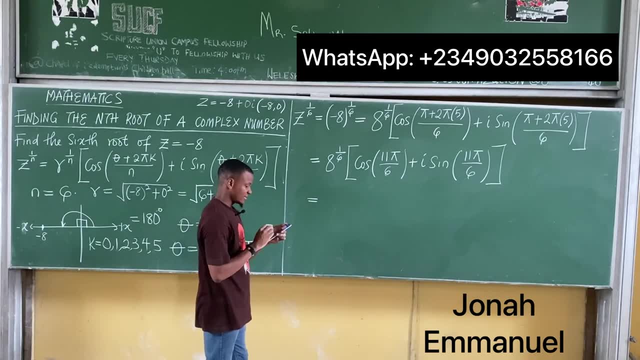 you want to. we can choose to get this answer in rectangular form. alright, so this will now be equal to: if I punch h to power 1 over 6, that gives me root 2 as my answer. okay, next up. so. 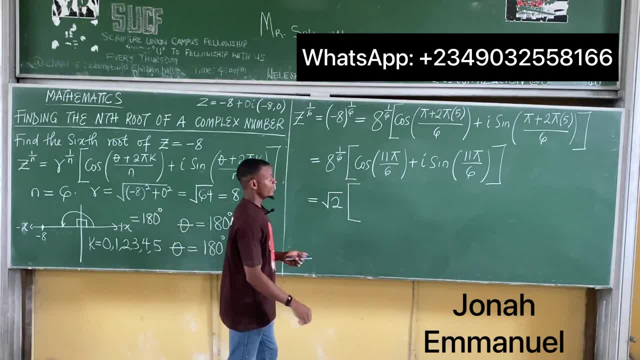 don't forget that we have this one here in radians because of the pi. so first of all convert your calculator to radian mode. then in radian mode punch cos, cos, 11, pi all over 6, so the answer there becomes root 3 all over 2.. 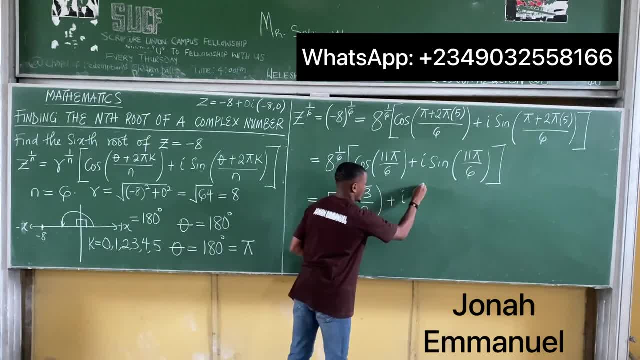 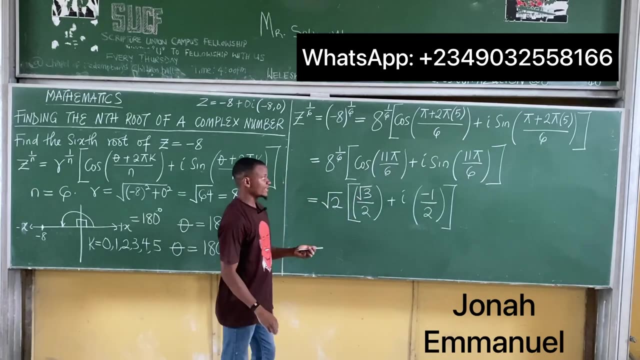 Plus I um punch sine this value, that's sine 11 pi over 6, that gives me minus 1 over 2, so I have this answer, Please. if your calculator is in degrees and you punch this, you probably will not. 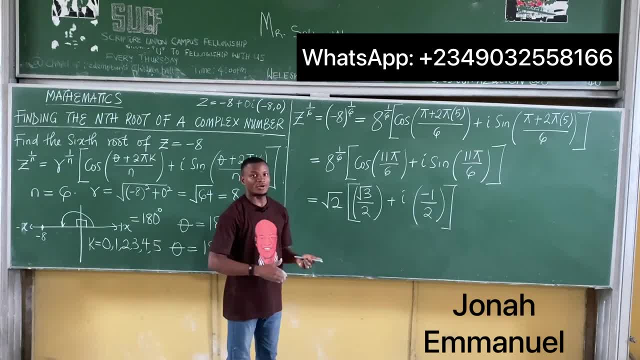 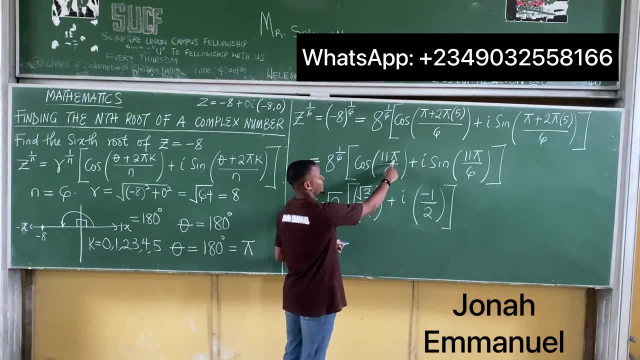 get these values. So your first task is to put your calculator in radian mode first before you punch them or simply convert to degree first. This pi will be equal to 180, so it becomes 11 times 180, all over 6,. now you take cos. 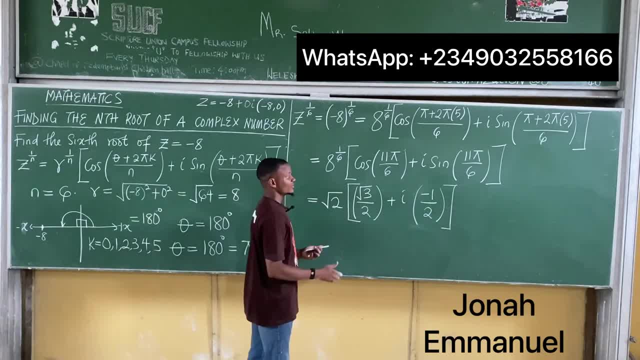 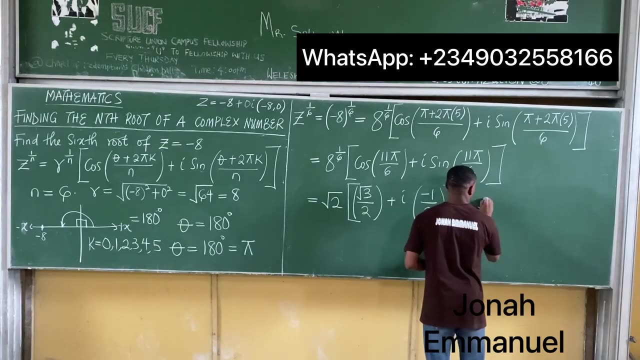 of that value. you have this, alright. or, better still, since this is in, since this is pi, put your calculator in radian mode, alright. change it to radian and then punch this. you have this value Alright. so that's equal to um. work on this. this becomes root 2 into um. I'm having this.